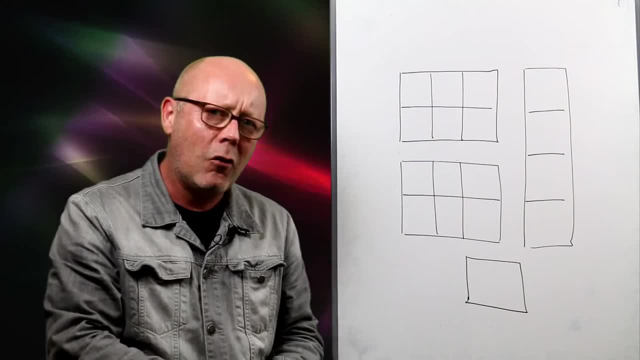 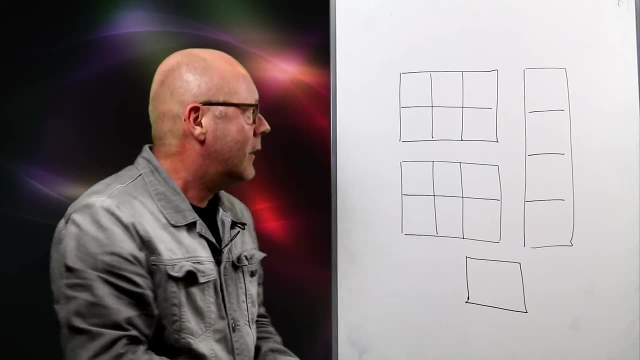 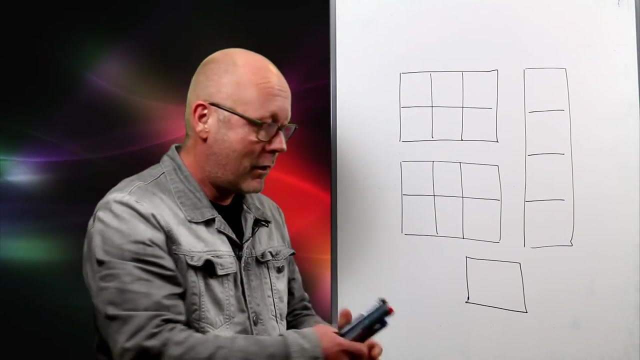 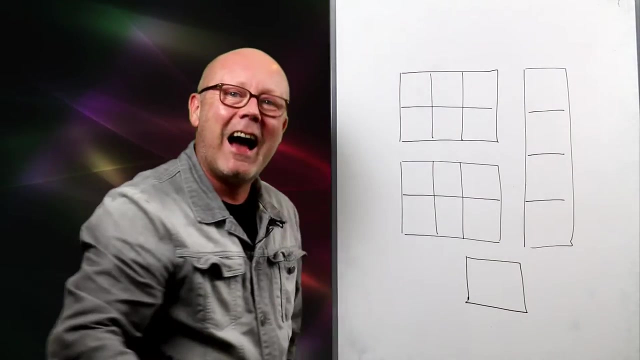 in a big soup and you can be a bit confused. So the goal of this video is to kind of clarify what are all these different things? right Here you see 17 empty boxes. We are going to fill them up. The first six boxes are called. In the first six boxes I'm going to put some quarks. 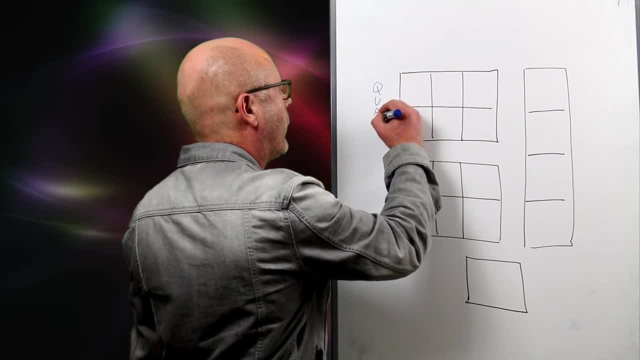 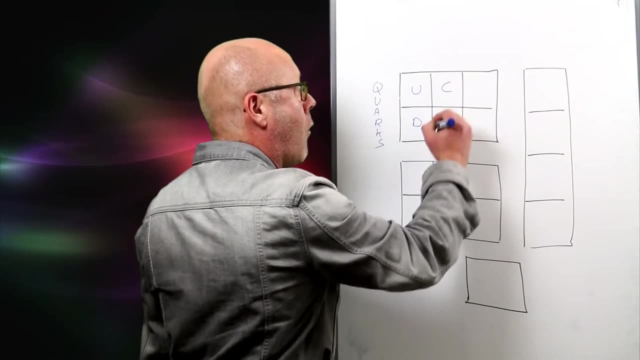 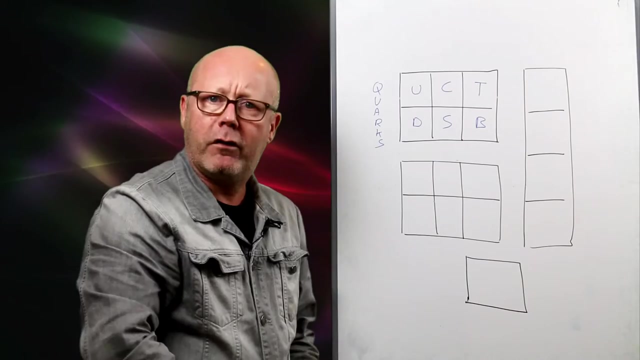 The up quark, the down quark, the charm quark, the strange quark, the top quark and the bottom quark. What are quarks? Well, you are familiar with neutrons and protons, which make the nuclei of atoms. Actually, 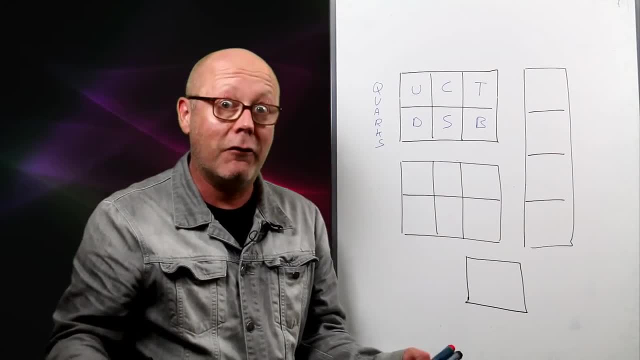 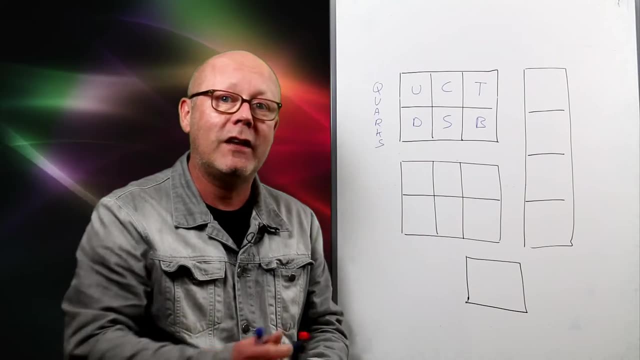 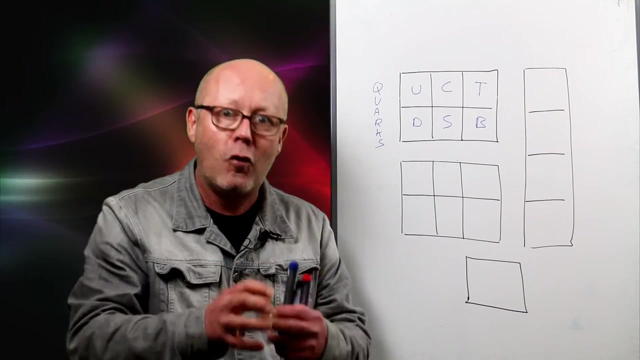 you know that all nuclei of all the atoms in the universe are made of neutrons and protons. But neutrons and protons are themselves made of quarks, which are tiny elementary particles. An elementary particle is a particle. you cannot break into smaller parts. Quarks are elementary particles. 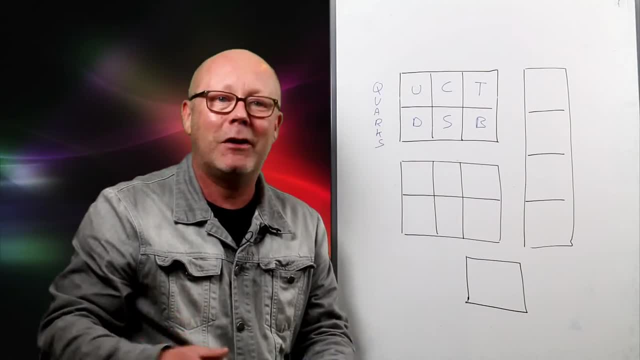 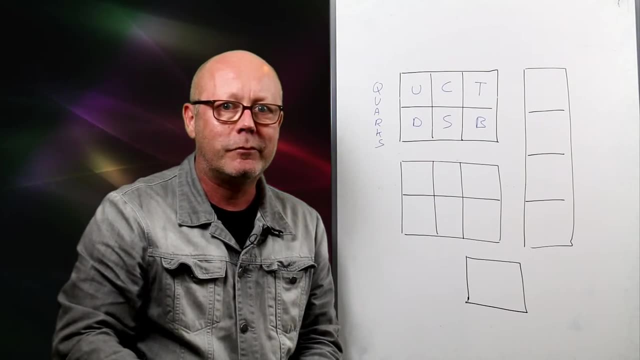 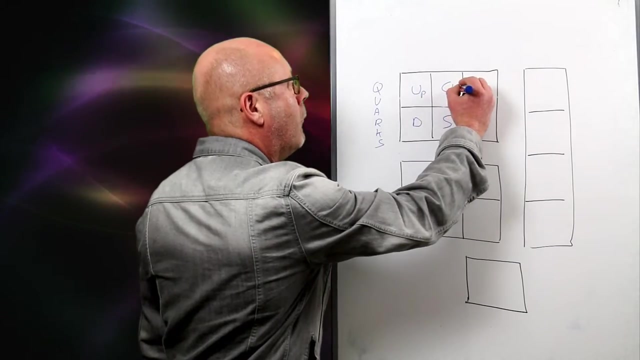 So basically the quarks make most of matter because the nuclei in an atom, you know it, kind of concentrates most of all the mass of the atom. So how to remember these names? Well, the up, the charm and the top are kind of positive type of quarks. 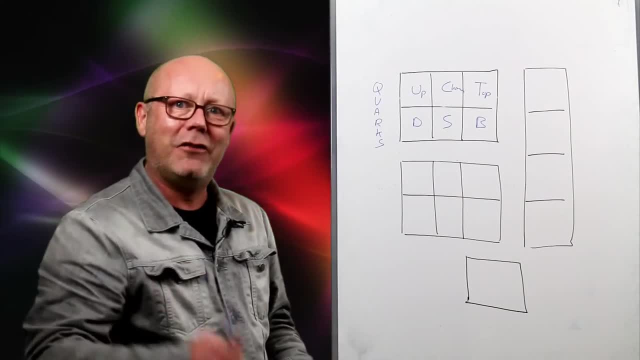 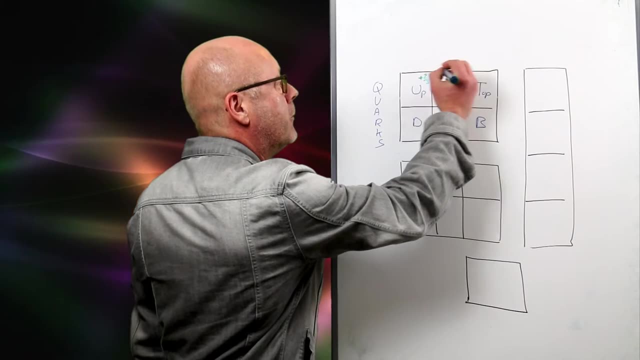 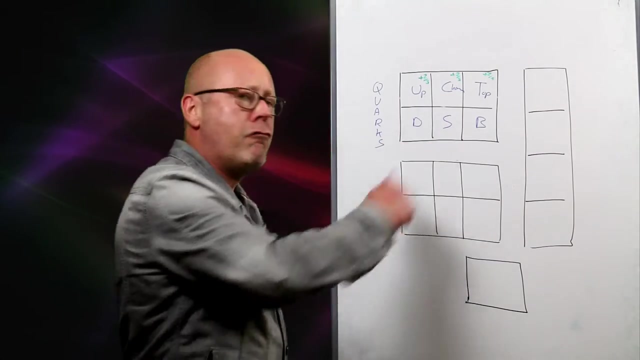 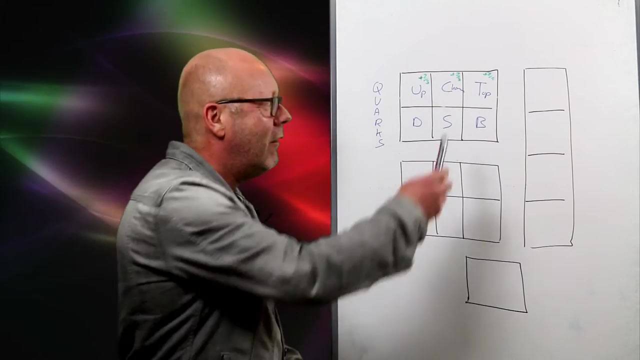 it's up, it's charming and it's top successful. So these quarks have got a positive charge which is plus two thirds of the elementary charge E. The low row is made of the depressed quarks Down. strange, a bit freaky, you know, bottom. 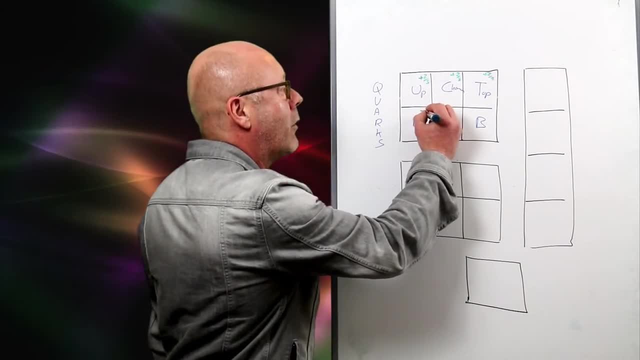 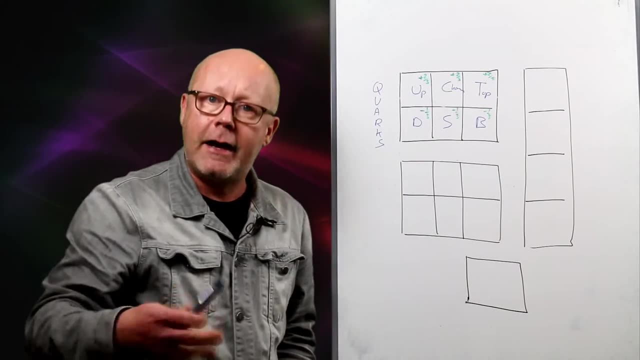 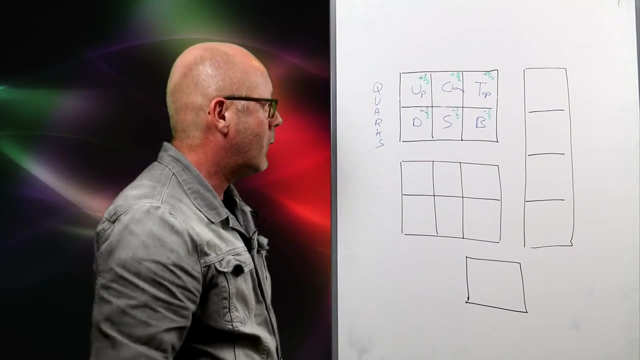 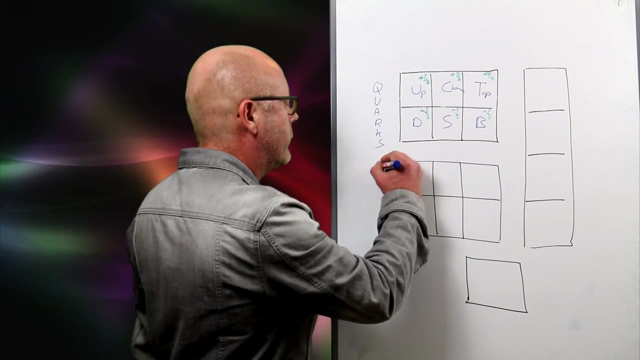 So these quarks will have a negative charge minus one third. Now these quarks can combine and create hadrons, but we will discuss this once we've filled up the whole table. The low six boxes are leptons. You know one lepton, the electron. 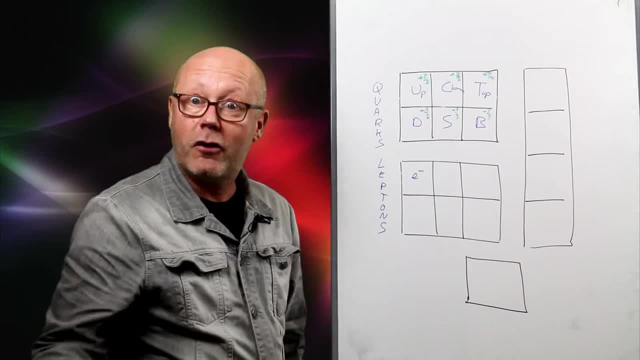 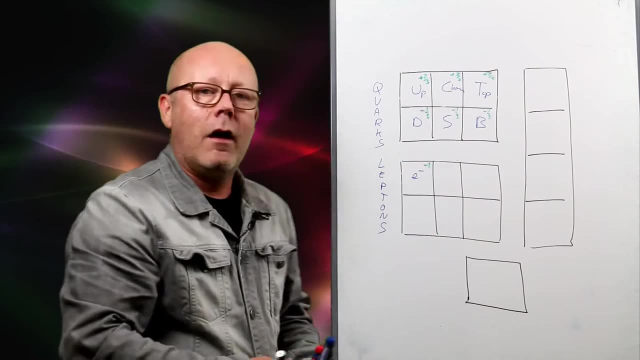 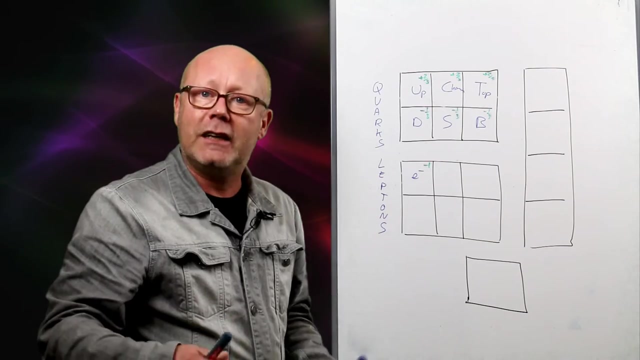 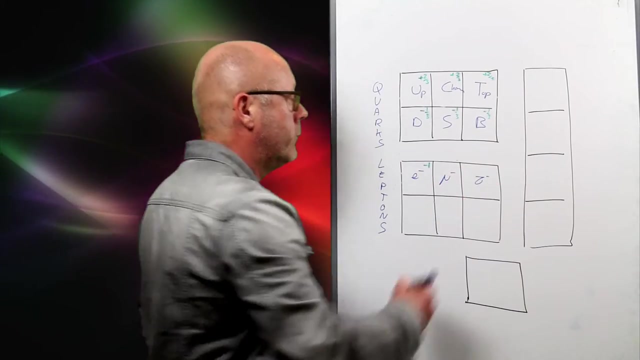 So it's got a negative charge, right. One negative charge- Let's write it down- Minus one. Well, the electrons has got cousins which behave exactly like electrons, but they are just of larger mass. These are called muons and top. Both have a charge of minus one. 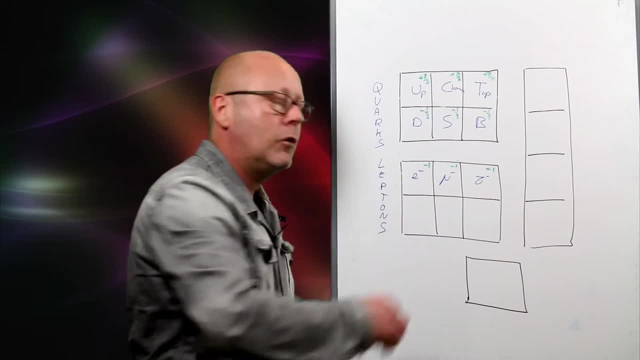 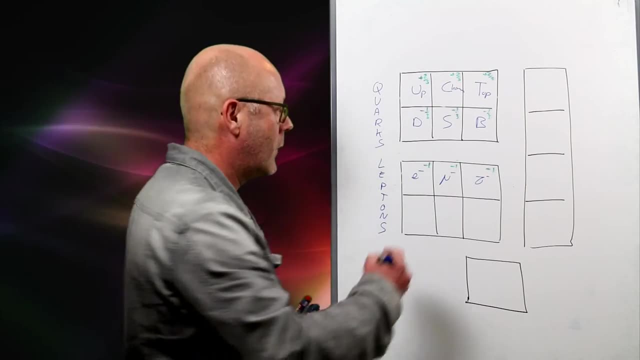 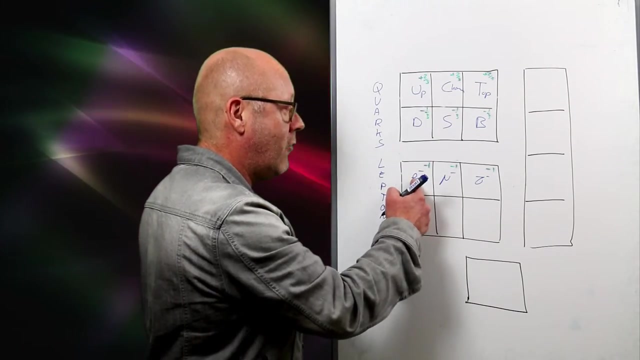 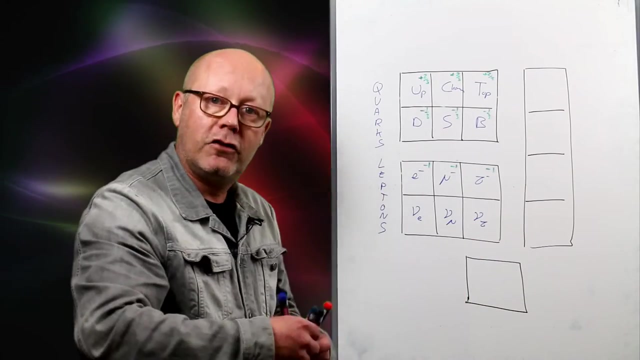 And here, what do we have? Maybe you remember in beta decay that you have neutrinos, which are formed. Neutrinos are also leptons and they come in three flavors: The neutrino of the electron, the neutrino of the muon and the neutrino of the tau. The charges of neutrino is zero. 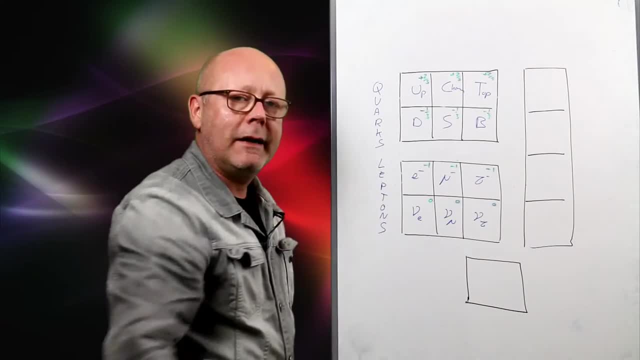 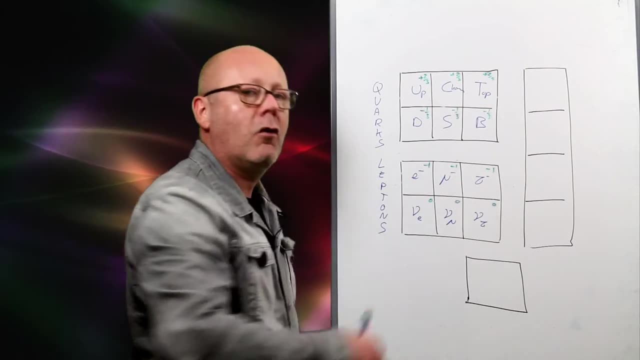 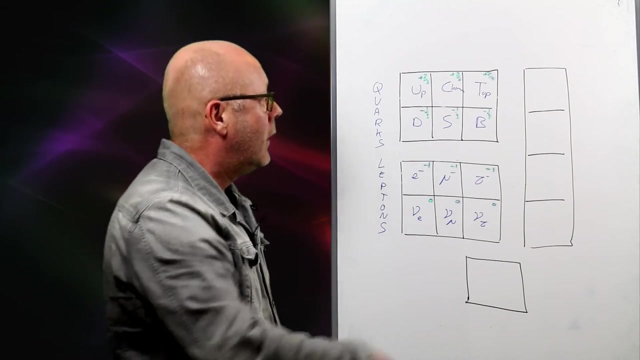 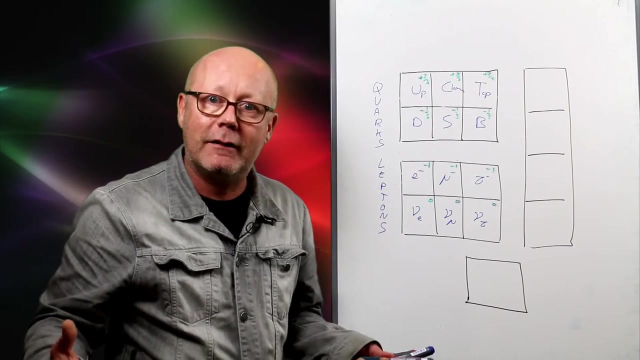 Now the quarks have large masses, the leptons have got small masses. In the lepton the electrons, muon and tau have got a small mass And the neutrino has got a very, very small mass. These particles are called particles of matter because they create the matter around us. 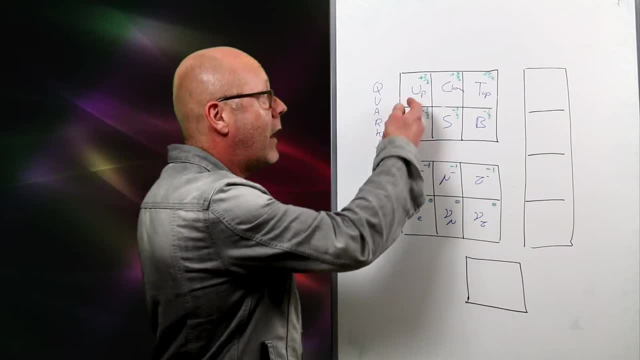 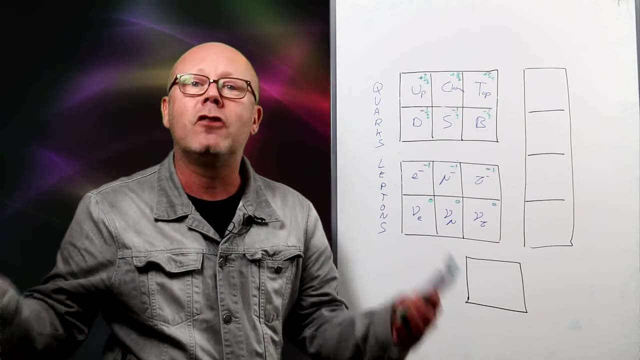 Take an atom, for instance. it's made of a proton, which is made of up and down quarks, and an electron, And the universe is also completely filled with neutrinos rushing around. We don't see them because they don't interact very much with 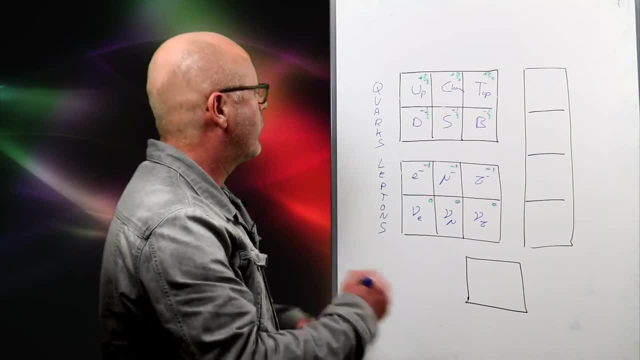 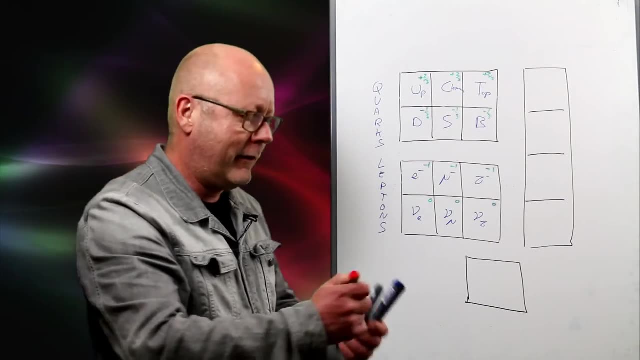 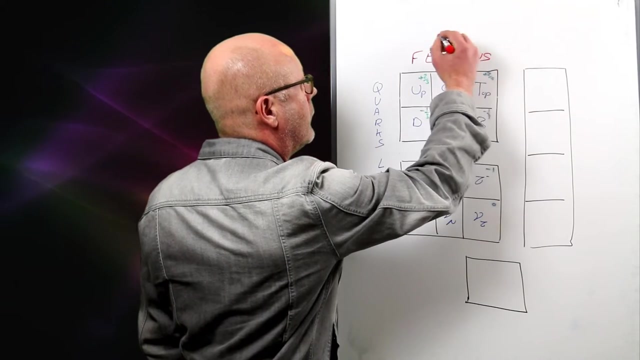 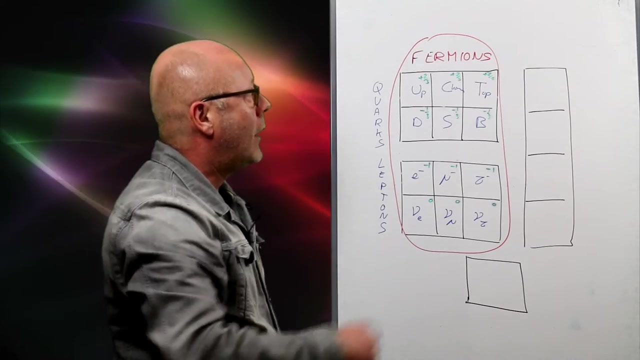 normal matter. So we like to group all these 12 particles as the particles of matter that we called fermions. I'm going to group them here up. These are the fermions. Why do we group them as a family, the fermion family? Because there 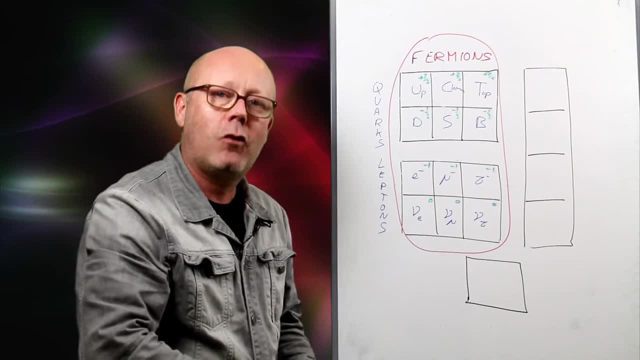 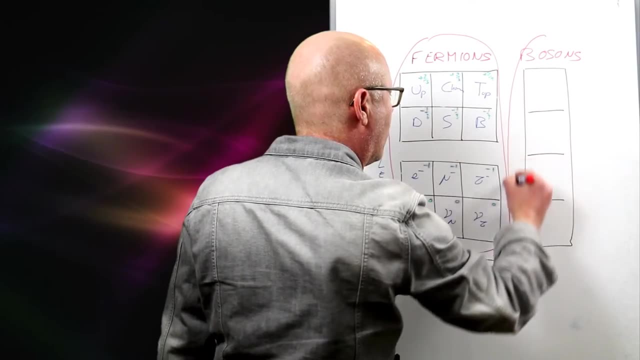 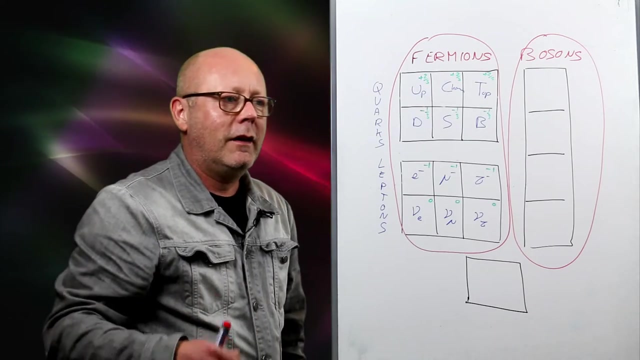 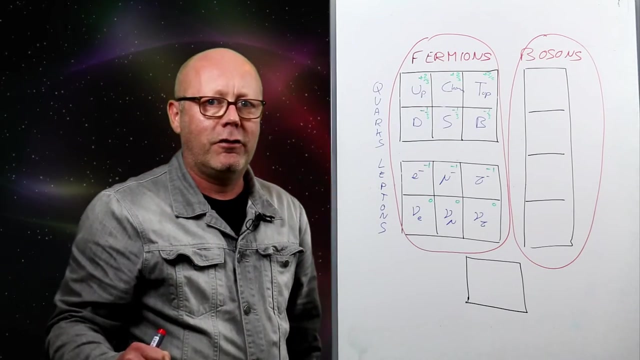 is another family here. This family is called bosons. You heard maybe that bosons are particles of force. It's a little bit difficult to grasp, But I'm going to give you a very simple example. Imagine two electrons. When you put the two electrons together, well, they will repel. 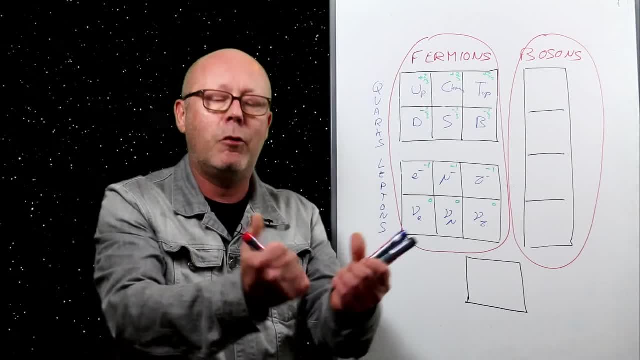 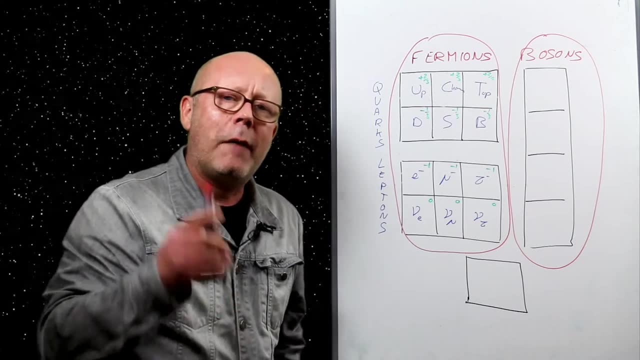 So there will be an electrostatic force, a coolant force that pushes them away from each other. But how does it really work? I'm going to use an analogy: Just imagine a bodon of air. And if you see the boon of air in the middle of a body, 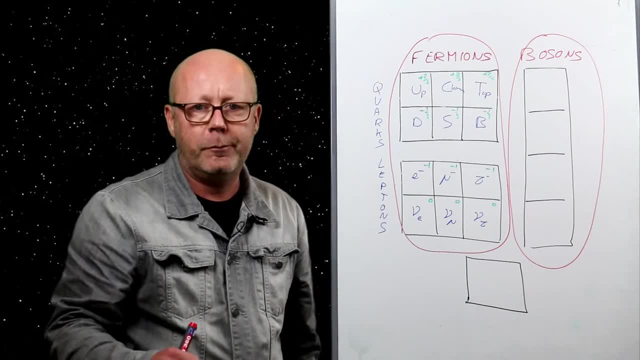 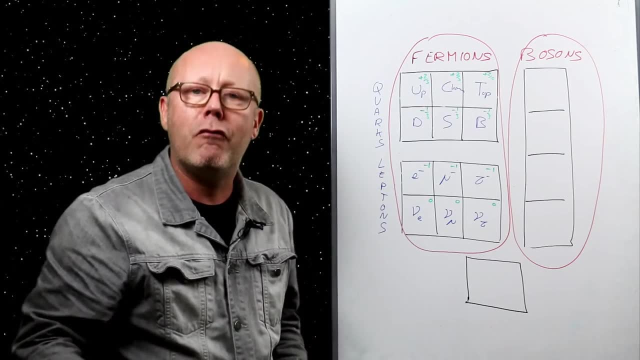 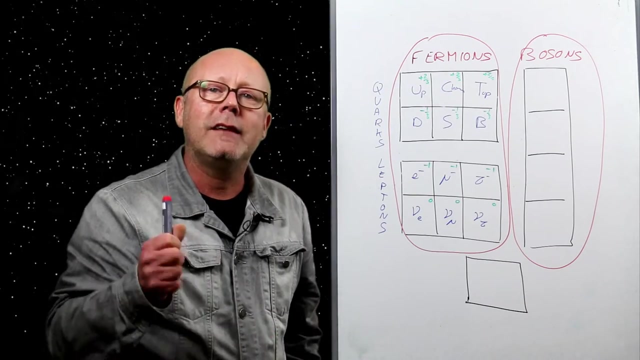 imagine a lake and on this lake there are two boats and on these boats there are two men, but the men forgot to bring a motor or the rows so they could move around. the two boats are stuck on the lake, but one of the men has a ball with him and he has an idea. he calls the other man. 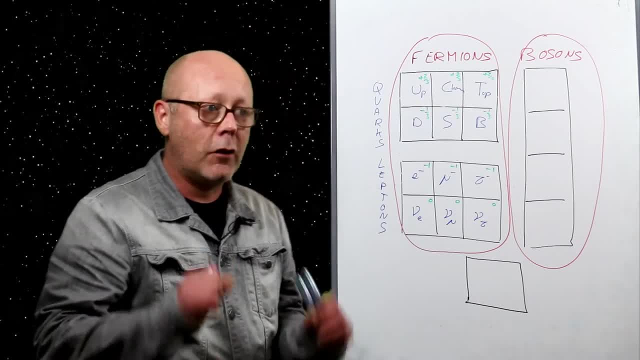 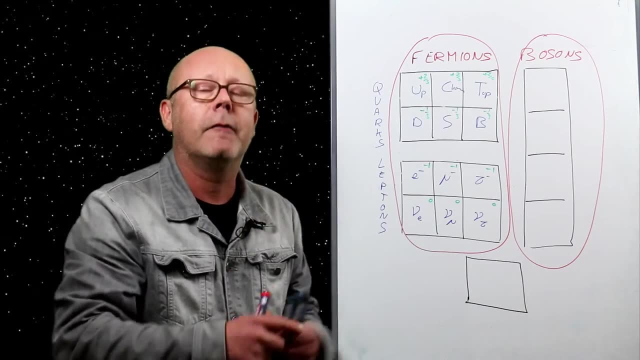 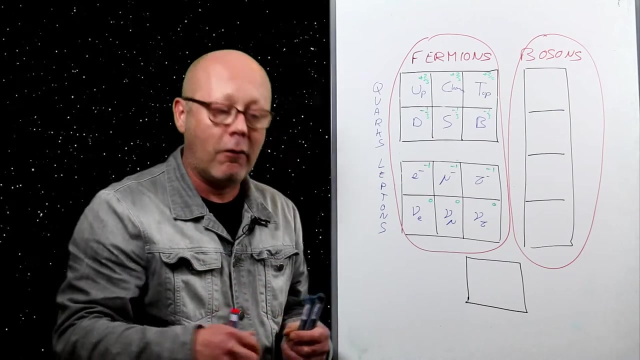 and he says i'm going to send you the ball. so he throws the ball to the other man, the. so the second man receives the ball and throws his back. now, each time one of the men throws a ball, there's a recoil effect on him and the boat while he throws the ball. he will. 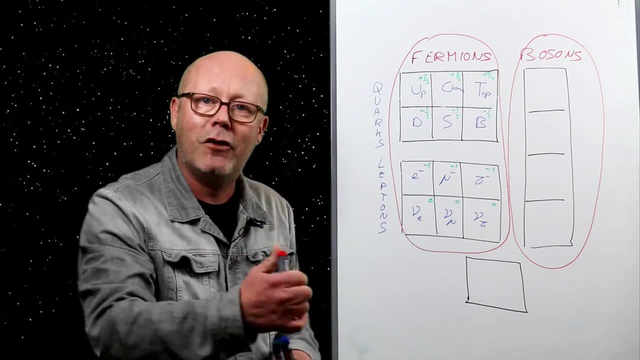 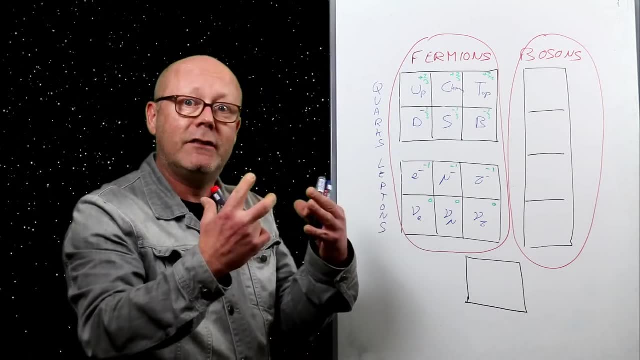 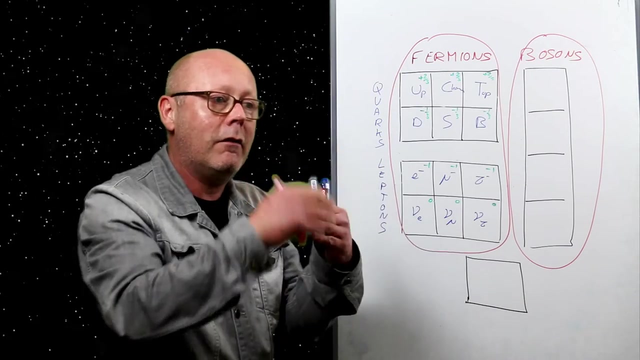 go backwards with the bow, the momentum of the man will change, and when the men receive, the other man receives the ball. well, he receives it, so his momentum will change too. he will also go backwards. so if they exchange a ball enough in a many times, they will actually appear like going away from. 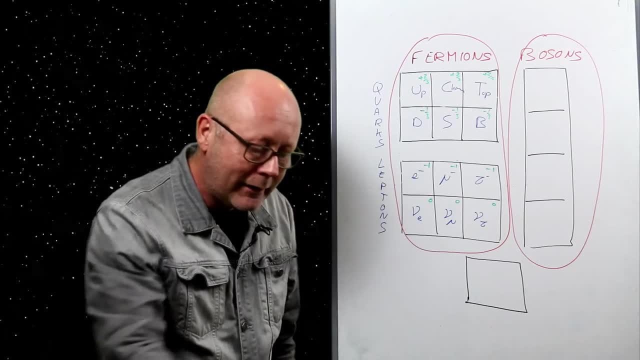 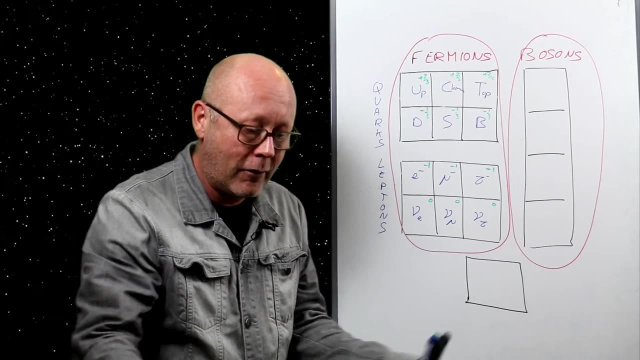 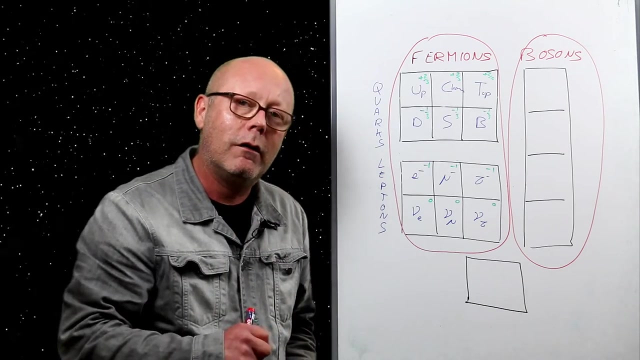 each other. now, if you look this from a plane, you might see the two boats, but you won't see the ball because it's too small. therefore, you see the two boats going away from each other and you think, oh, the two boats are repelling each other, while the ball is the particle of force it's called. 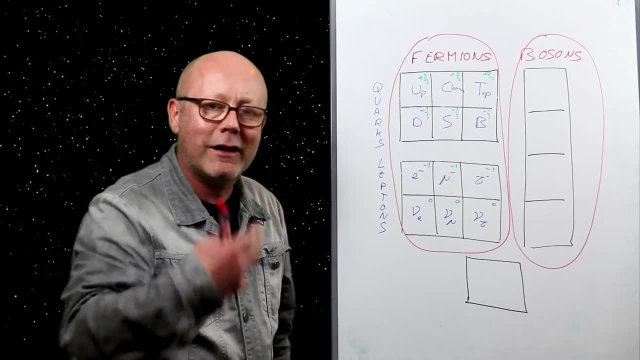 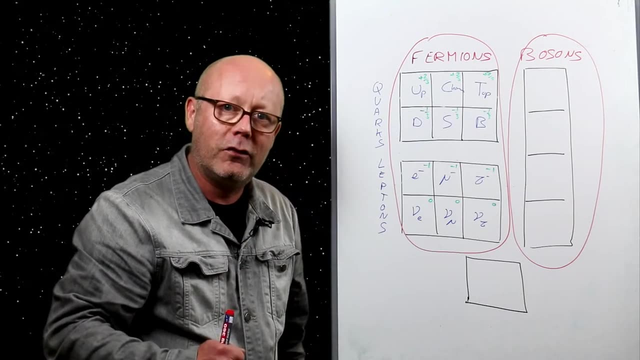 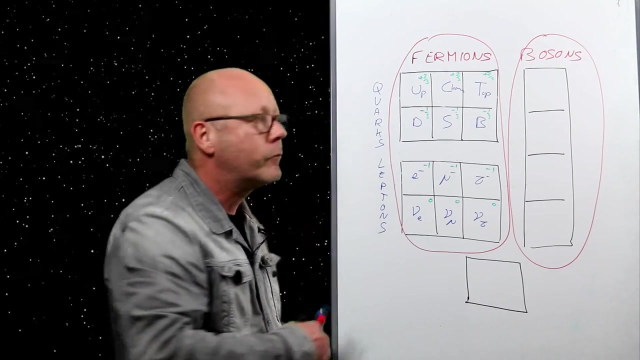 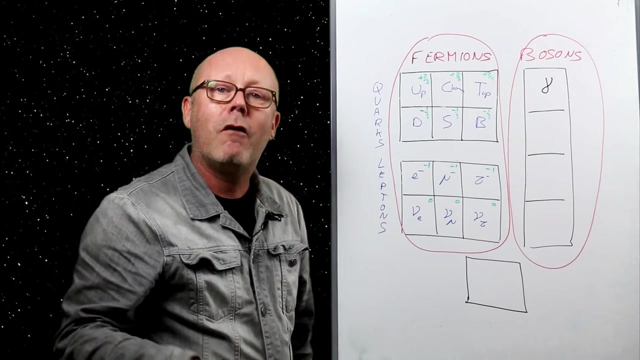 the exchange particle, because the two boats, or two particles, like the electrons, will exchange a boson and for the electromagnetic force, ie the coulomb force. here this particle is a photon. yes, the particle of light, the photon, is the exchange particle for the electromagnetic force. 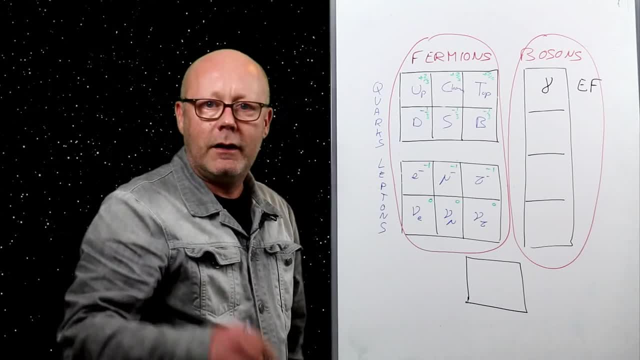 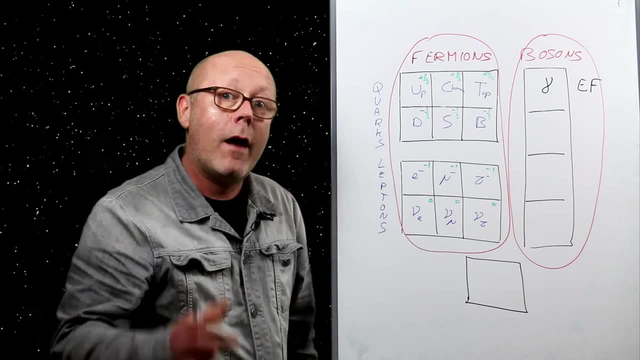 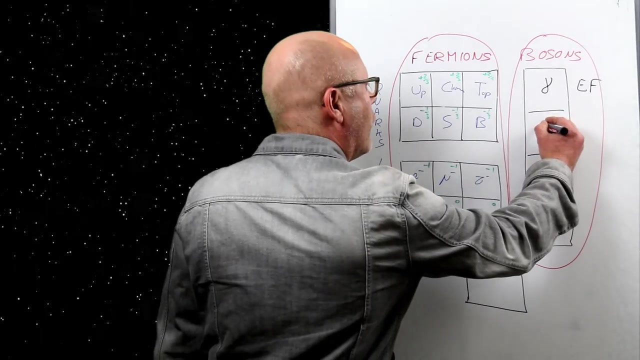 now you know there are four forces in nature: the electromagnetic force, and you've seen, in nuclear physics there was also a strong force where actually the quarks are held together by exchanging gluons. the gluon is the exchange particle or the boson of the strong force. 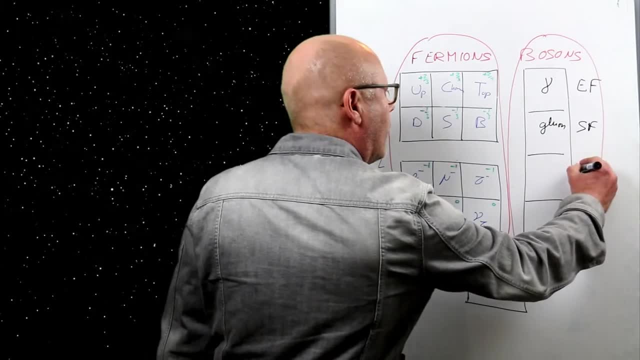 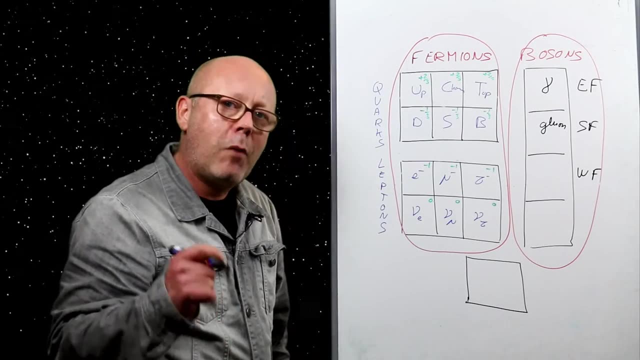 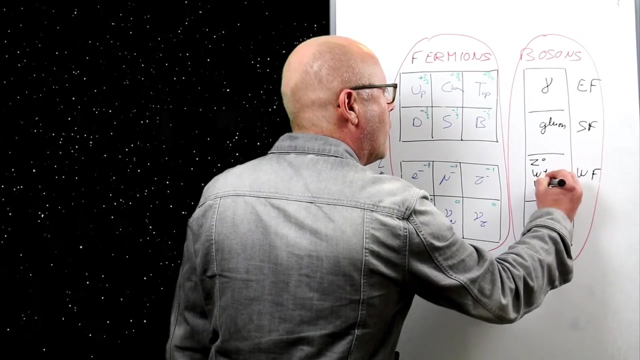 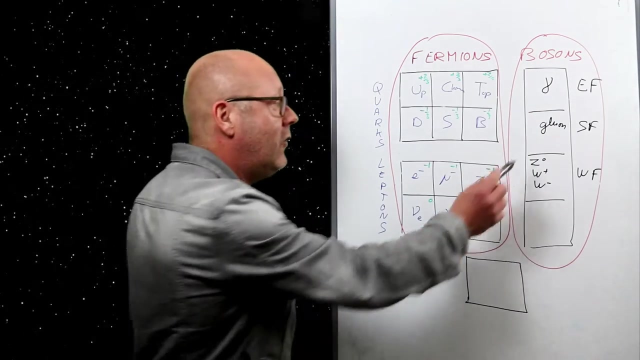 there's another force called the weak force, involved for instance in beta decay. now the boson of the weak force come in three variations: z zero, w plus and w minus. well, these, the photon and the gluon, do not have mass, but these do so. because they have mass, they have inertia and they cannot travel at the speed of light. they travel slowly. that's why the weak force is not able to travel at the speed of light. so the gravitational force has a very short range and finally you have the gravitational force, and the gravitational force would be carried by gravitons. but this is still an hypothesis, because gravitons have never been observed. 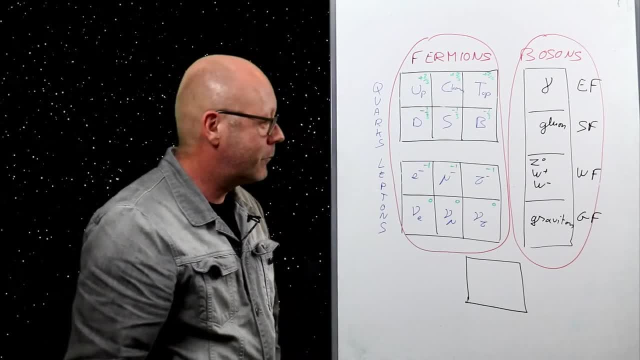 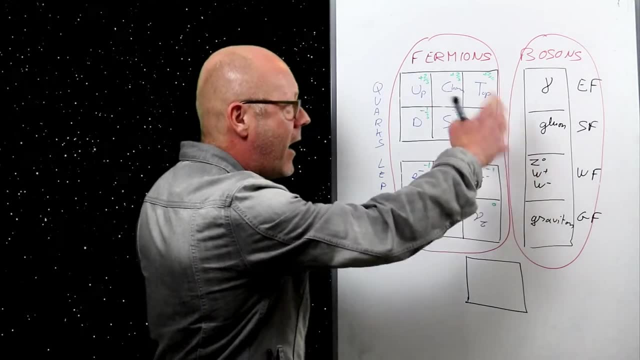 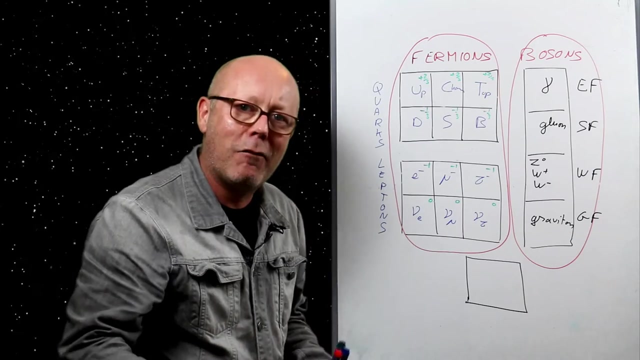 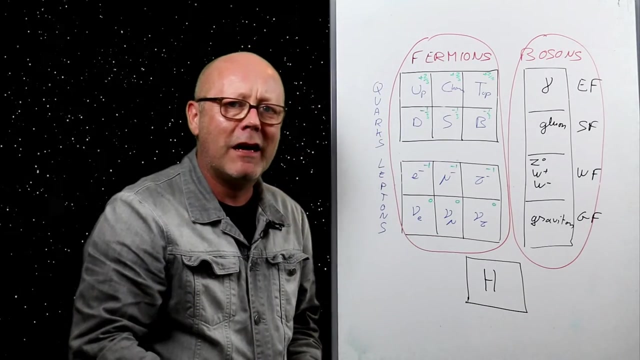 so we have now 16 particles. good, well, what's in here? in here there's a special type of boson. it's not really an exchange particle. it's a particle that provides mass to the other particles, the higgs. now, how does it provide mass to other particles? by interacting with them or not? 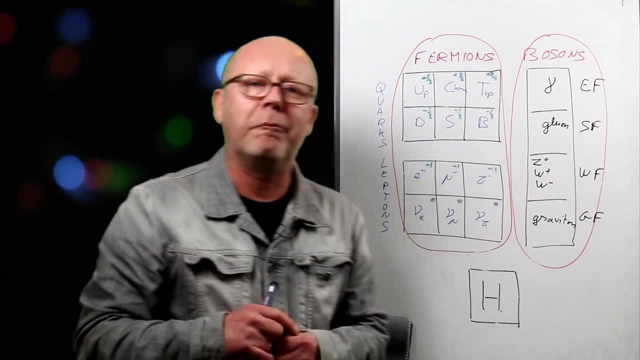 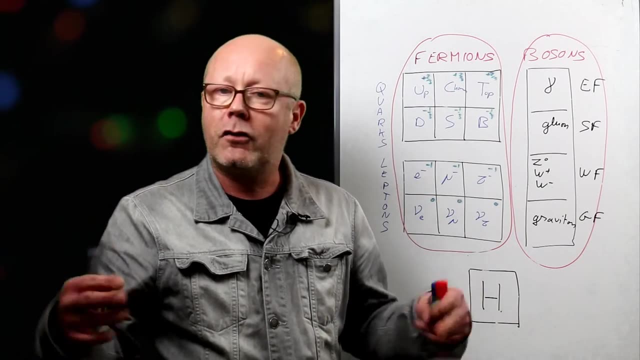 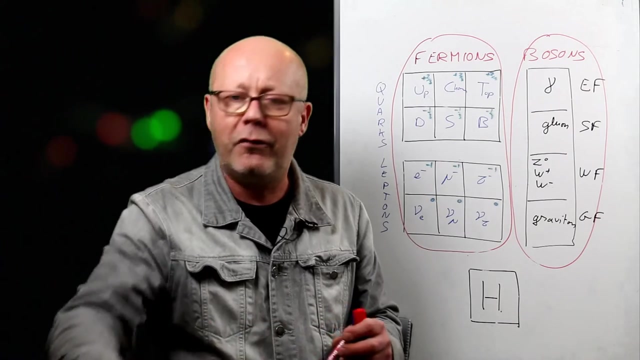 in order to understand this, let's let me tell you a little story. imagine a conference with lots of scientists and after the conference they all join and gather for some socializing after a hard day's work in a town hall where there's a buffet with some drinks. 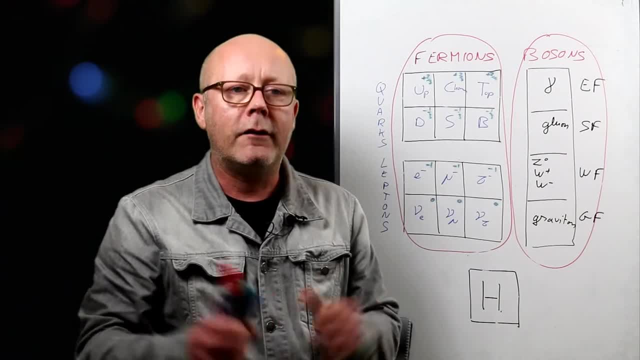 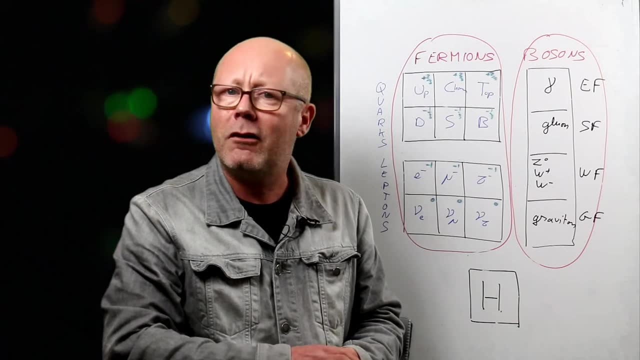 on the other side of the room there's a big door, and through the door arrives a man, a tax inspector. well, i don't know about you, but i don't really like tax inspectors. so i wouldn't talk to him, and neither would either the scientist. so 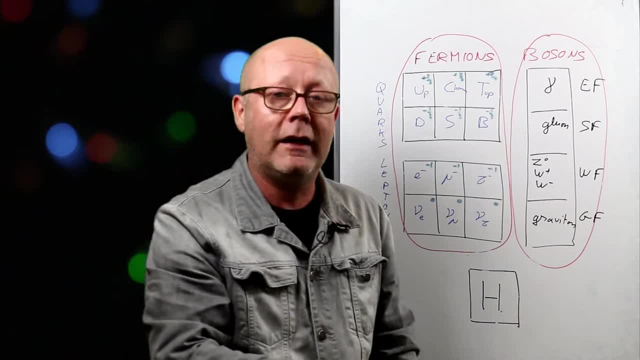 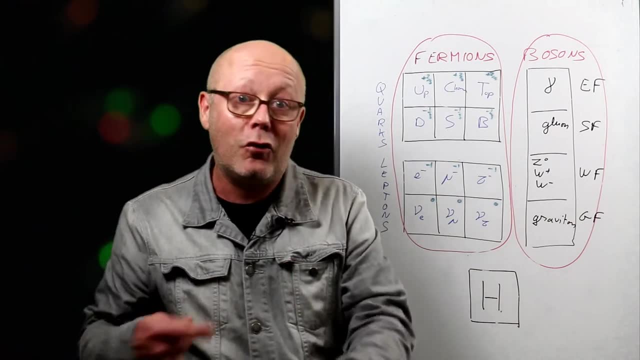 So the tax inspector, he's thirsty, he goes straight to the buffet, and well, at the buffet he gets his drinks Well. so he was able to go to the buffet at the fastest pace possible. A few minutes later, another man enters the door. 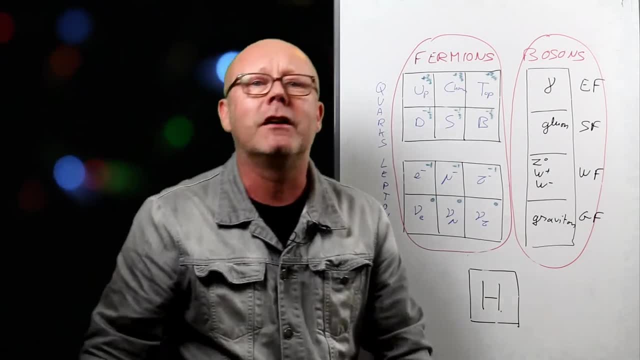 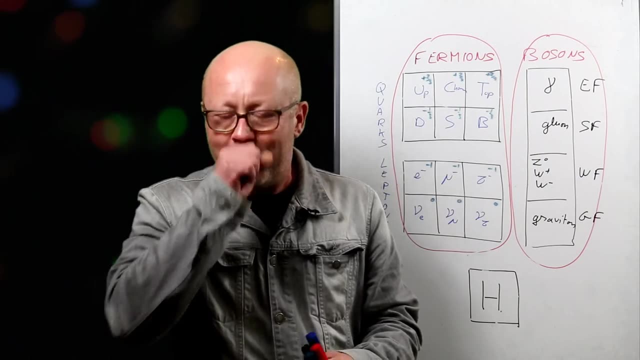 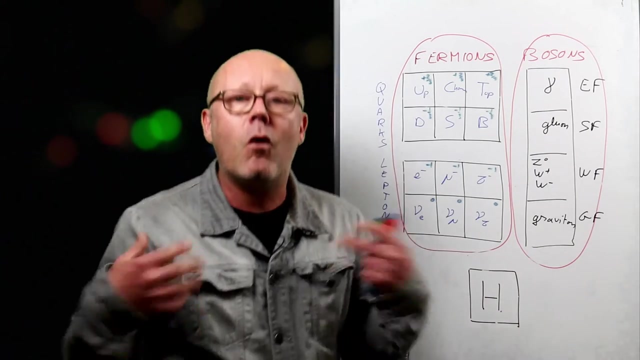 This man is Albert Einstein. He revived and he decided to pay a little visit to his colleagues on Earth. So he opens the door. and, of course, all the scientists Albert Einstein. they all want to talk to him, So they just all gather around him. 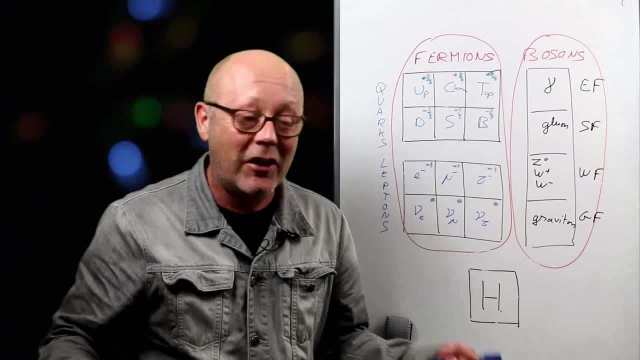 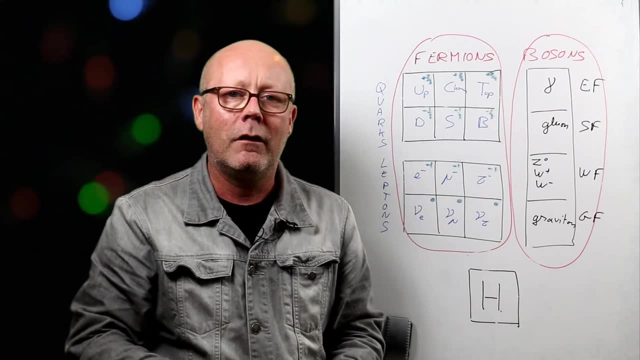 But Einstein, he just wants a drink too. So he tries to go to the buffet, but he can't. He's always blocked by all these scientists trying to talk with him. He's blocked by all these scientists interacting with him. So this analogy- 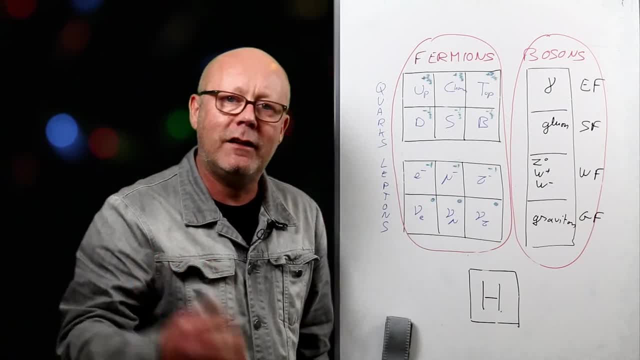 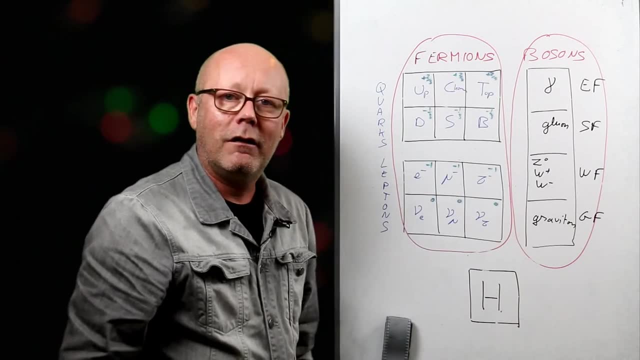 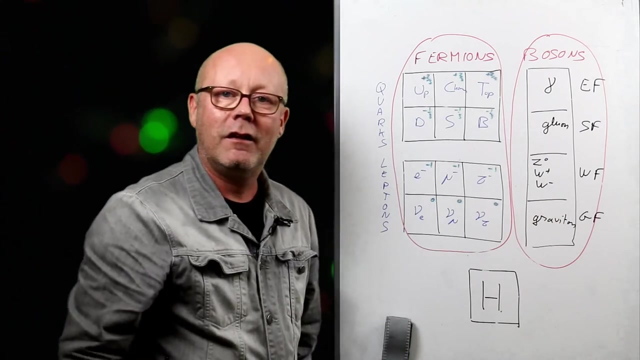 This analogy brings us back here. The scientists are the Higgs boson. Einstein is something like the top quark for which the Higgs boson interacts a lot, But the tax inspector is like the photon: He can go straight to the buffet. 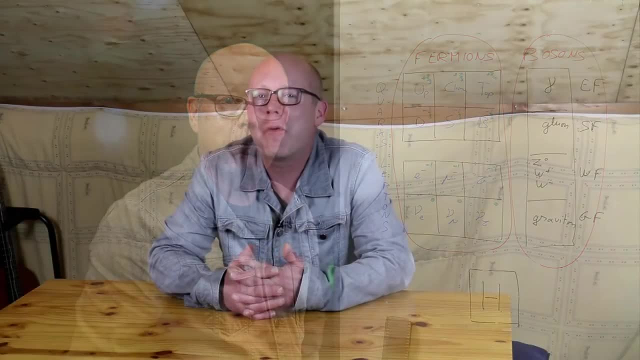 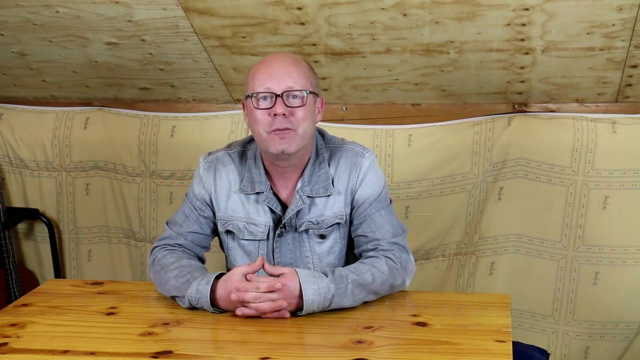 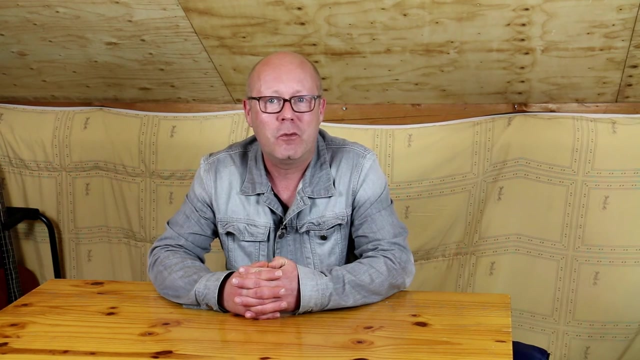 The photon goes at the speed of light. So with this little story, we have seen how the Higgs boson provides mass to the particles. It interacts more or less with them. Now space is full of Higgs bosons. More precisely, we call it the Higgs field, a field filled with Higgs bosons. 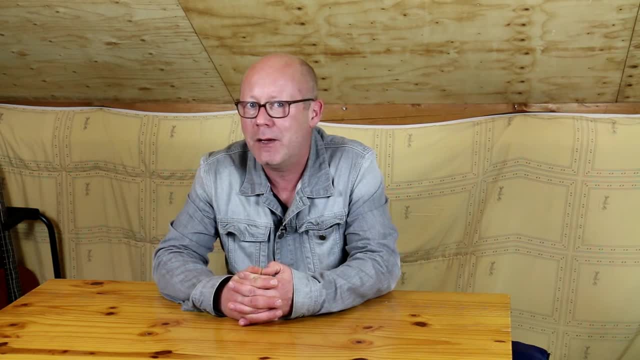 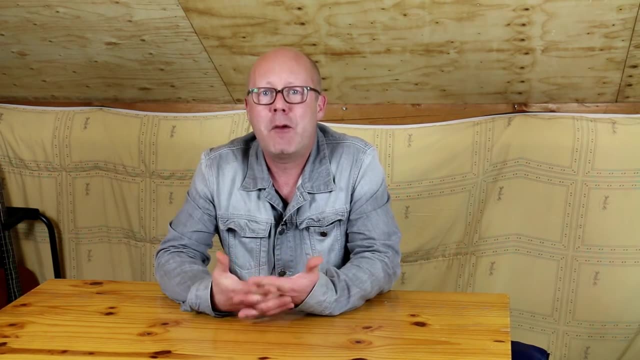 So when you're actually walking around, you are walking around billions and billions and interacting with billions and billions of Higgs bosons. Now, the top quark is a very heavy particle. That is why it interacts a lot with the Higgs boson. 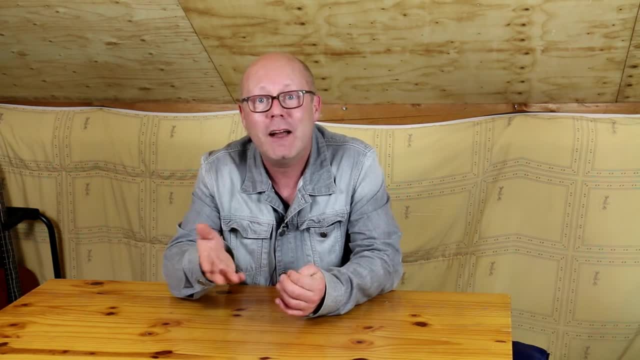 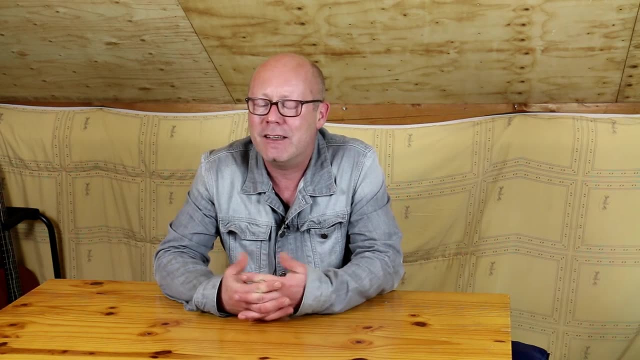 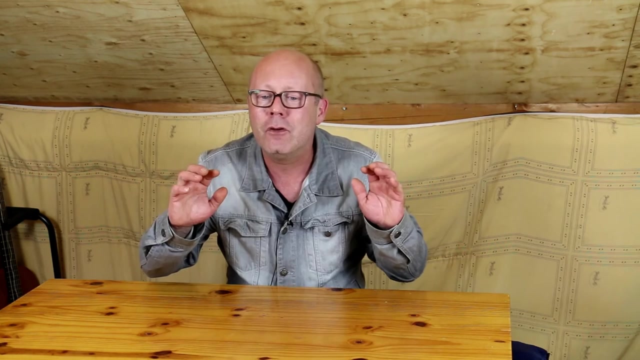 That was the example used for Einstein, which interacts a lot with the scientists when he's trying to go to the buffet. Think about it. Mass is force per unit acceleration, meaning that you need to bring a lot of force to the top quark to accelerate it a little bit. 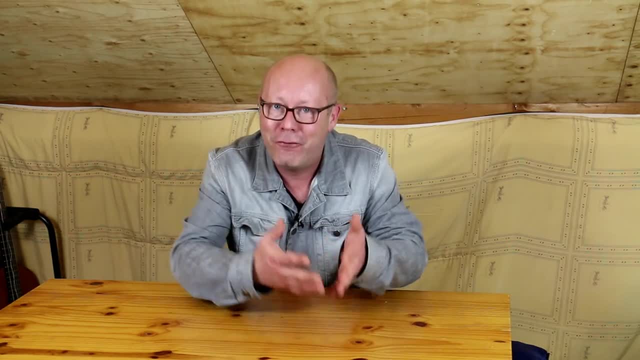 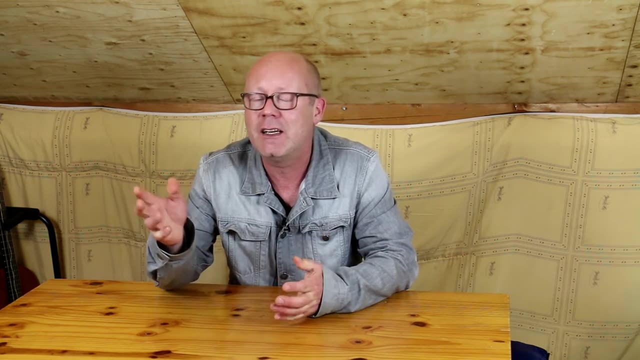 The top quark has a lot of inertia, which is due to the strong force, So it has a strong interaction with the Higgs boson. On the other hand, you can consider the photon that we've seen, like the Texan specter.